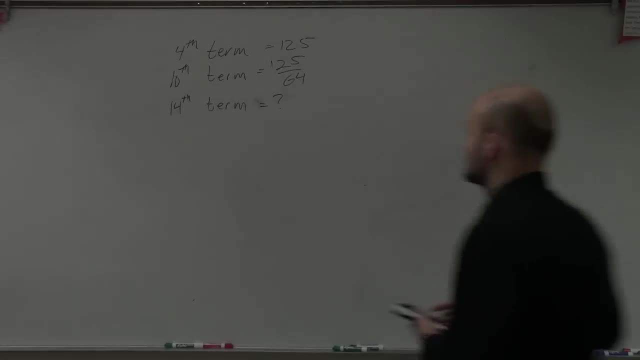 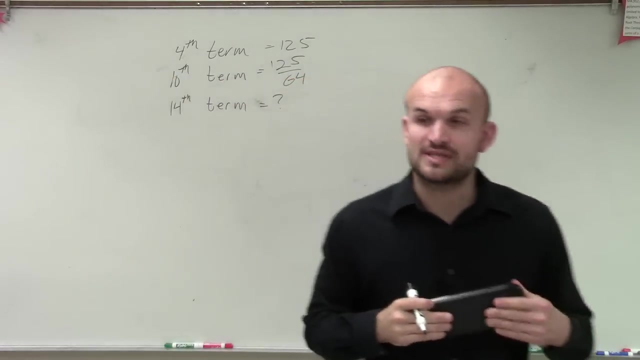 Okay, just let me go through this real quick. So we have the fourth term equals 125,, the 10th term equals 125 over 64, and they want us to determine the 14th term. alright. So obviously, ladies and gentlemen, we're trying to find an nth term. right, We're not talking. 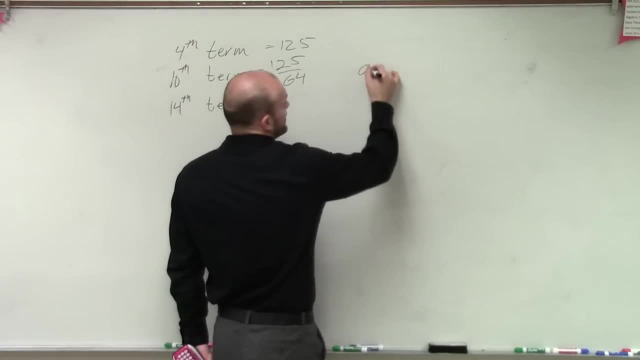 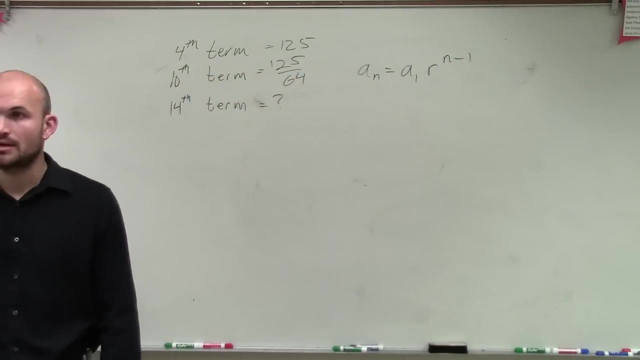 about sums. so, therefore, we know that the formula we're going to have to use is: a sub n equals a sub 1 times r to the n minus 1,. right Now, all I want to go through, ladies and gentlemen, is when we're looking at something like this. remember when we talked about arithmetic? 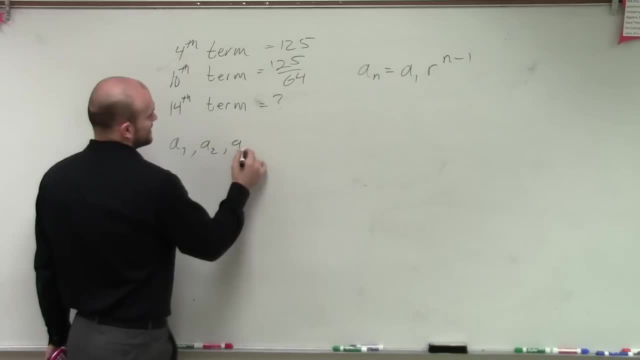 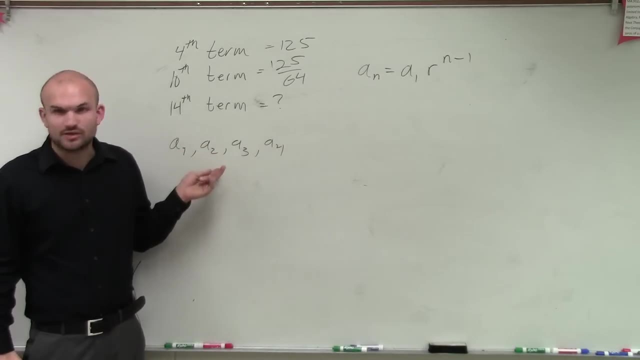 sequences: if I said a sub 1 times a sub 2 times a sub 3 times a sub 4, remember we said a sub 2 minus a sub 1 has to equal a sub 3 minus a sub 2, right, Those had to equal each. 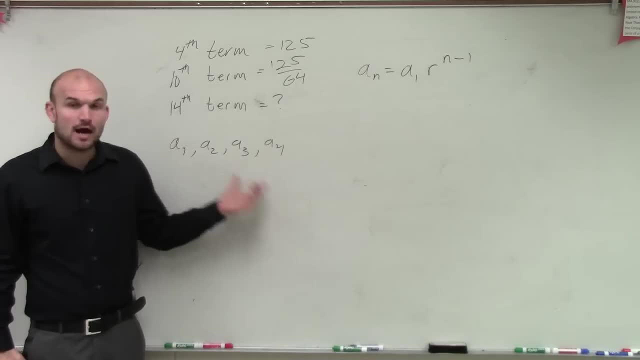 other right, And that equaled our difference. However, what if we weren't given a sub 2 and a sub 1? What if we were given a sub 3 and a sub 1?? We knew, though, that we can. still find the difference between a sub 1 and a sub 2.. So we're going to have to find a sub 1 and a sub 2.. So we're going to have to find a sub 1 and a sub 2.. So we're going. 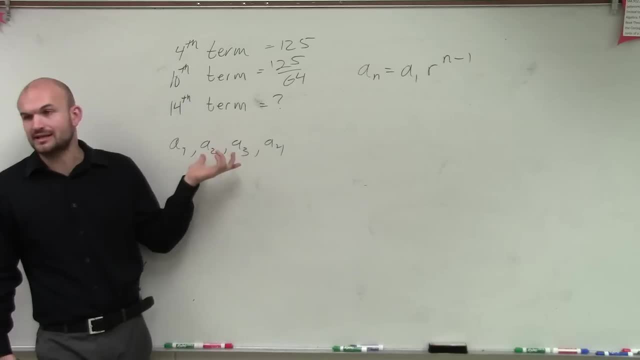 to have to find a sub 1.. So we're going to have to find a sub 1 and a sub 2, right, and that's going to be a sub 1 times 2.. We can argue: look that what we're going to. 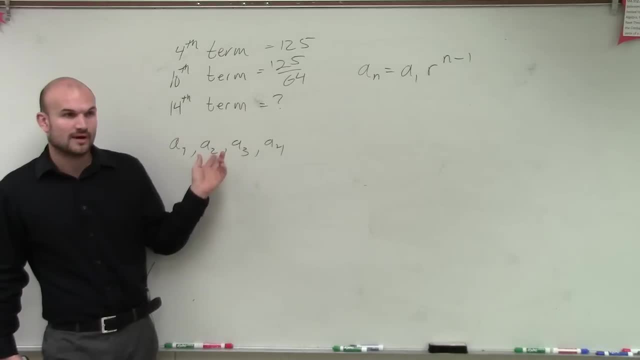 find is going to be a sub 3 minus a sub 2 minus a sub 1 times shell, a sub 3 times Nothing except a sub 2 plus a sub 3 minus a sub 2.. This 아이 exactly what I mean by. 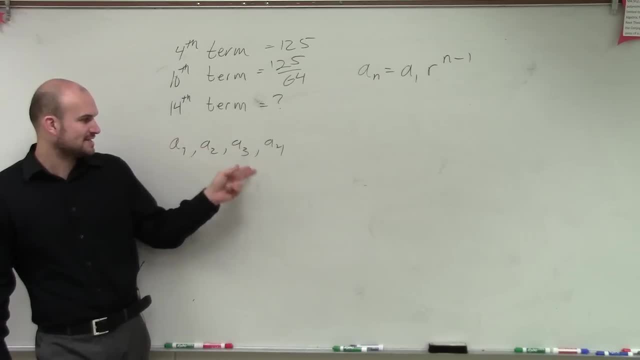 that, And then we're going to have to find the difference between these two values, which is going to give us our difference. However, if we know we have a common ratio, would the ratio then of a sub 3 over a sub 1? 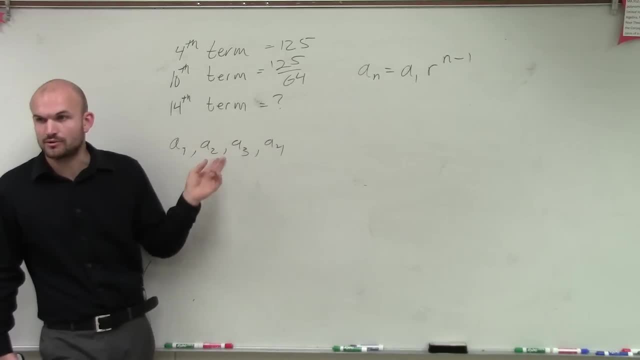 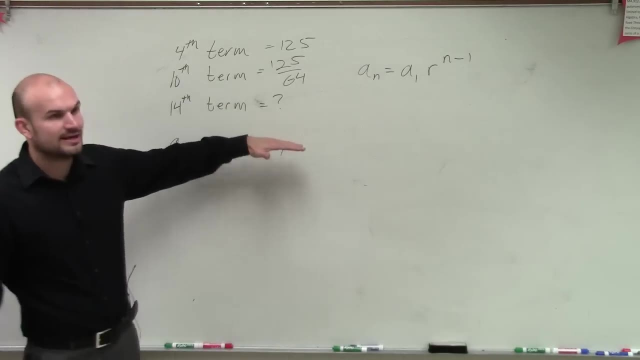 still be equal, with a sub 3 or a sub 4 over a sub 2?? It won't be our r, but would it still be our ratio. Would it still be equal ratio? Yes, So, ladies and gentlemen, what I can do then? 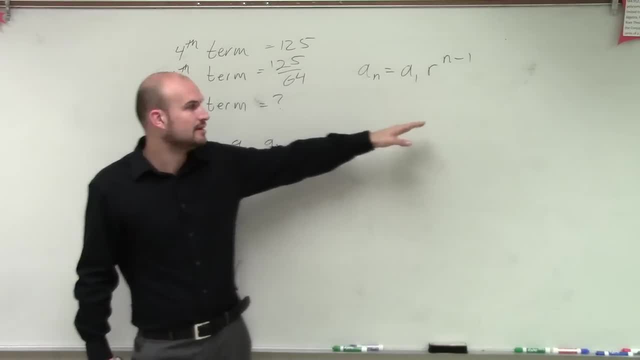 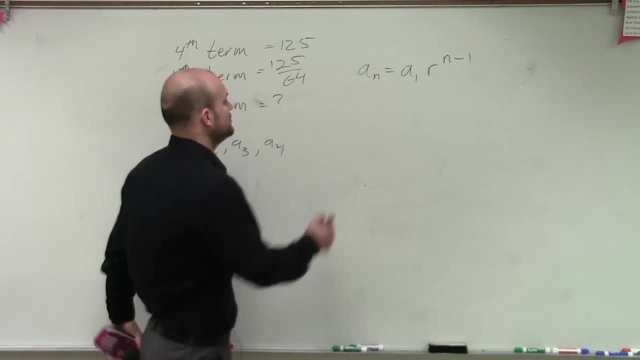 is, I can still apply the terms that we're given to be able to figure out what our r is, because that's what we need to do is figure out the r. So to do that, rather than we don't have a sub 1,. 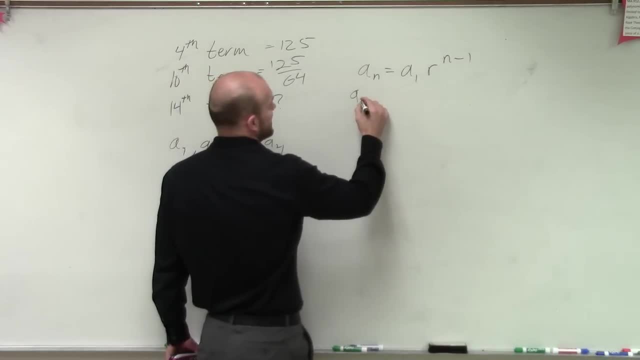 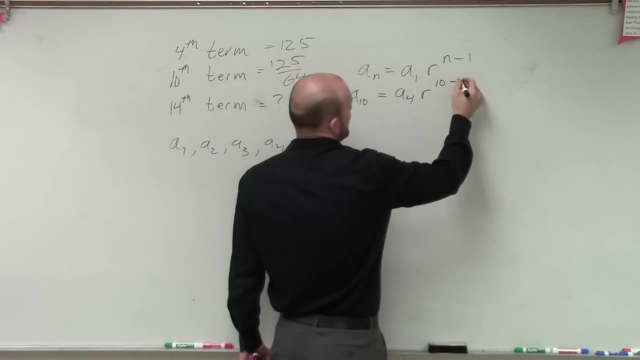 so let's just go and take this as our 10th term. So let's do: a sub 10 equals a sub 4 times r to the 10 minus 4.. So what I'm doing is I'm not starting at 1 and 1.. 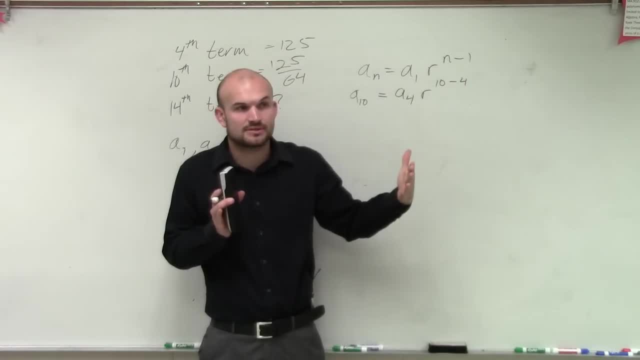 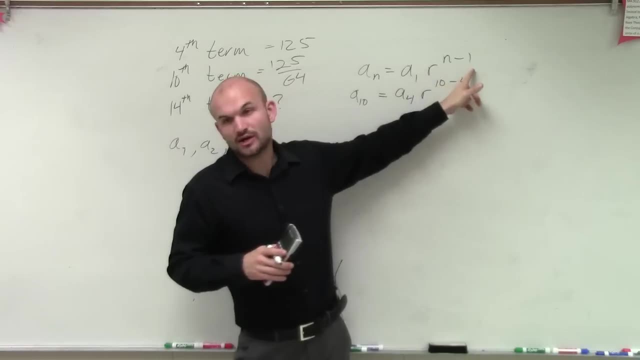 Now what I'm doing is I'm just finding the ratios between the two terms. That actually is going to help us now find r. Does that kind of make sense? Because we're not starting at 1.. It's a sub 1 and 1.. 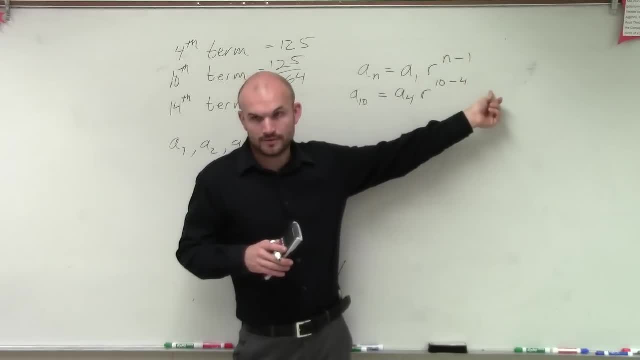 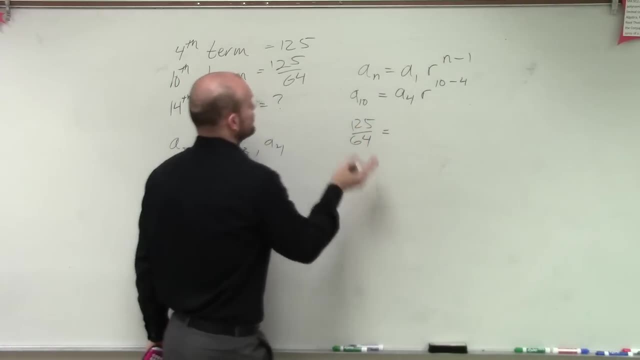 We're not going between 1 and 1.. We're going between a sub 4 and 4.. So now we know that a sub 10 is 125 over 64 equals a sub 4, which is 125, times r to the sixth power. 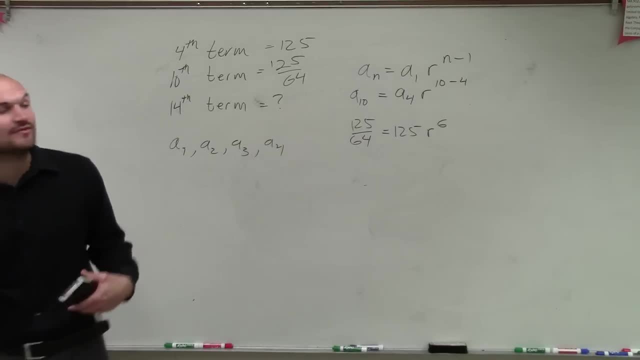 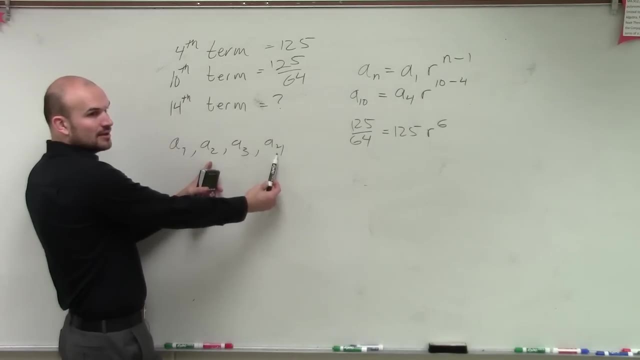 Now, by solving for r, by plugging in these two values and solving for r, I can find out what the exact ratio. so it's like me, given I have two values, But just dividing these two values is not going to give me my ratio. 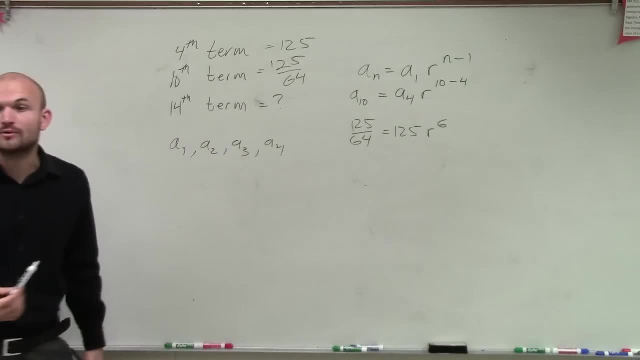 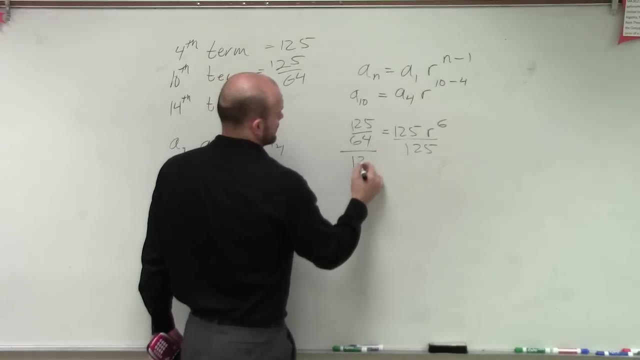 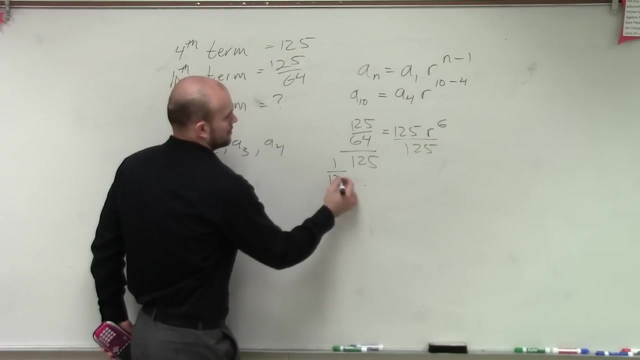 But if I plug them into the formula I can now find out what that ratio is. So now divide by 125.. Remember, taking a fraction divided by another number, you can multiply by the reciprocal. That will multiply that out to 1.. 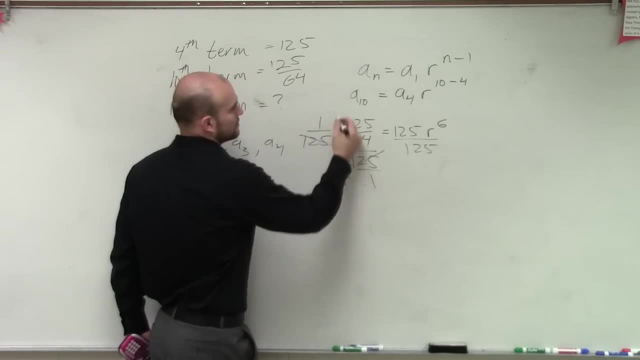 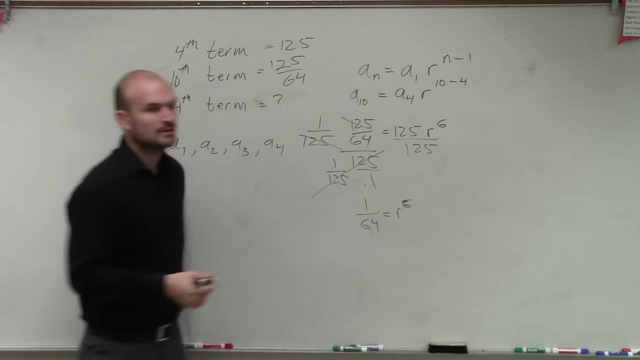 Multiply the top by the reciprocal That now divides out to 1.. So you're left with 1 over 64 equals r to the sixth power. So remember, just like when we had x squared equals 4, you took the square root of both sides. 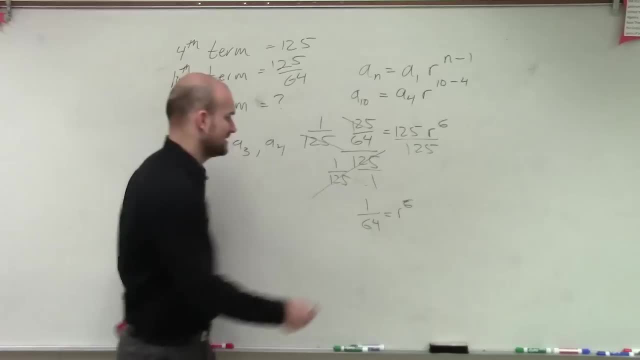 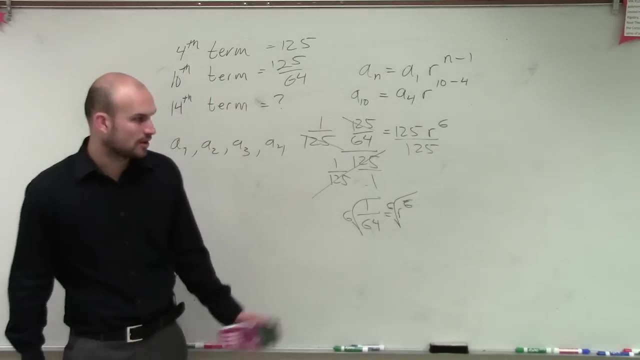 Now we have r to the sixth power equals 1 over 64. So we take the sixth root of both sides And then you say: what is the sixth root of 1 over 64?? Well, remember, we can break this up into sixth root of 1. 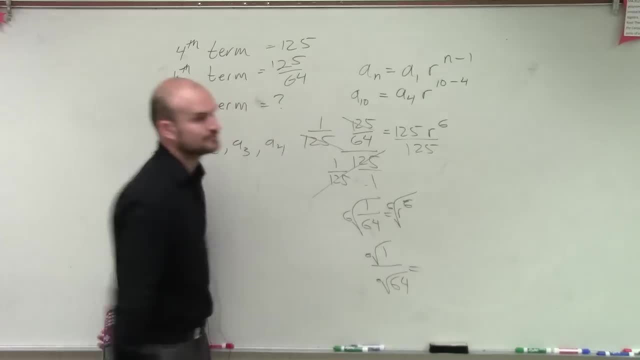 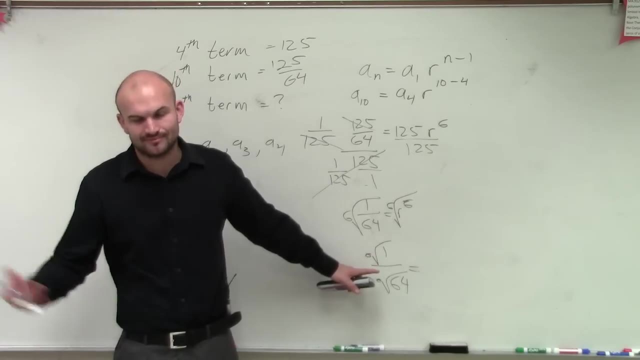 over the sixth root of 64. And you could say the sixth root of 1,. what number, multiplied by itself six times, gives you 1?? That's obviously 1.. What number, multiplied by itself six times, gives you 64?? And you want to first start and see. 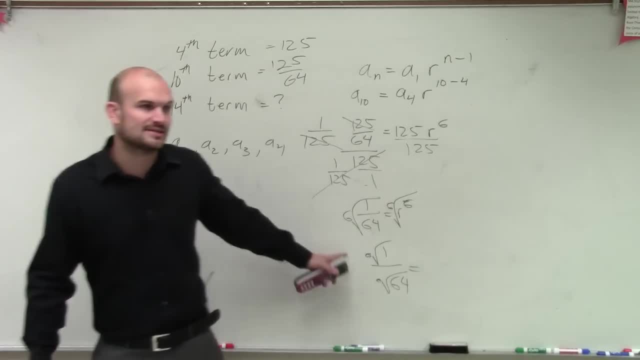 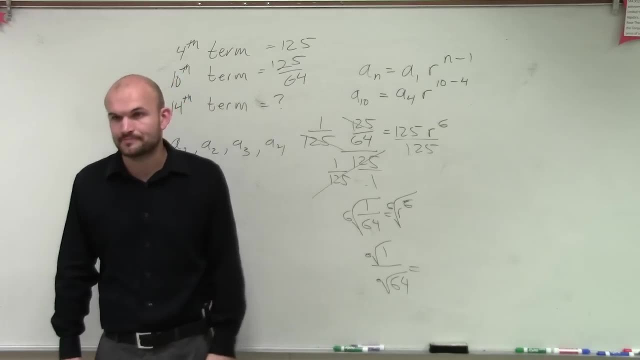 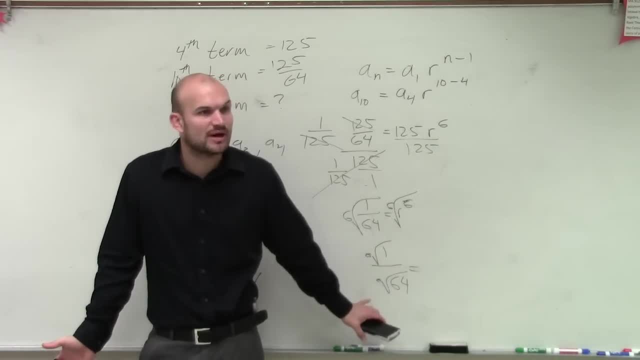 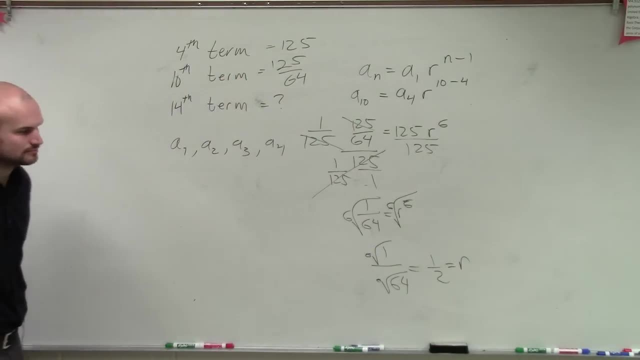 But yeah, You can plug it in your calculator Or you can just understand what number multiplied by itself six times, So you can see that our r is equal to 1 half. Wait, Is that supposed to be a 6 next to the number? 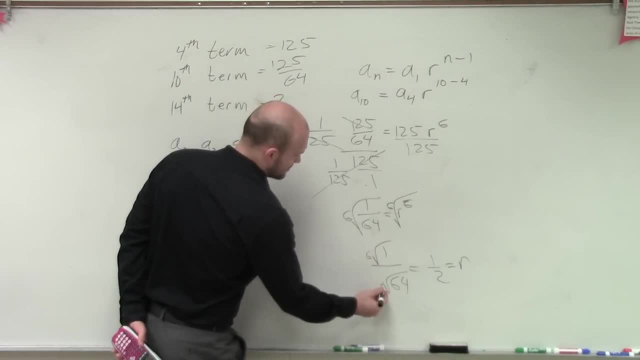 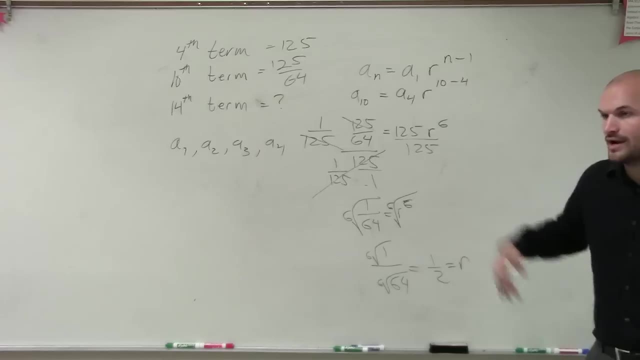 Yeah, It's a 6.. Come on, That's a beautiful 6.. What's 1 half? It's a beautiful 6.. So now we know our 1 half equals our r And we want to be able to determine the 14th term. 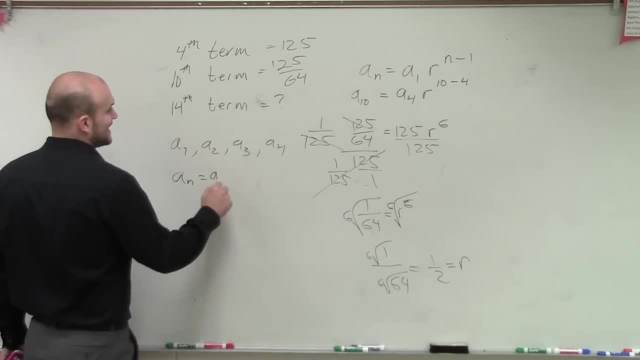 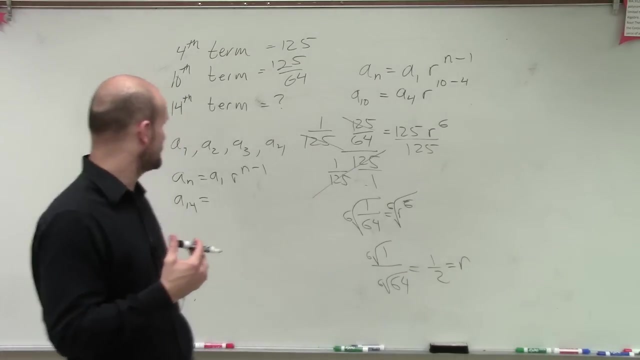 So now, ladies and gentlemen, if we have a sub n equals a sub 1 times r to the n minus 1, now, if I want to figure out what 14 is, I know what a sub 1 is not. So actually I need to go ahead and figure out. 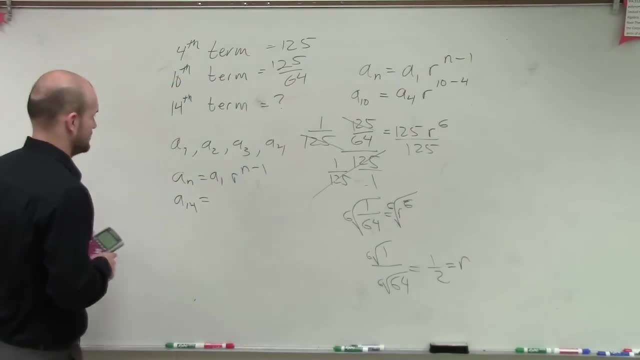 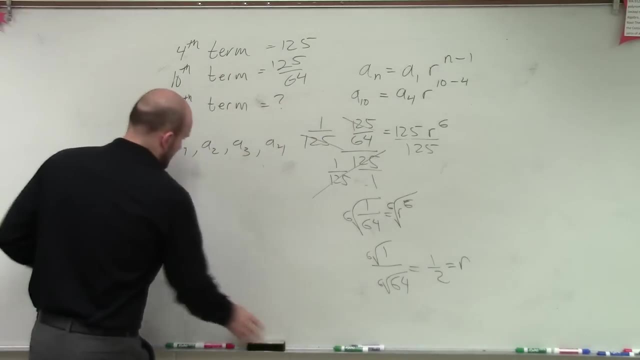 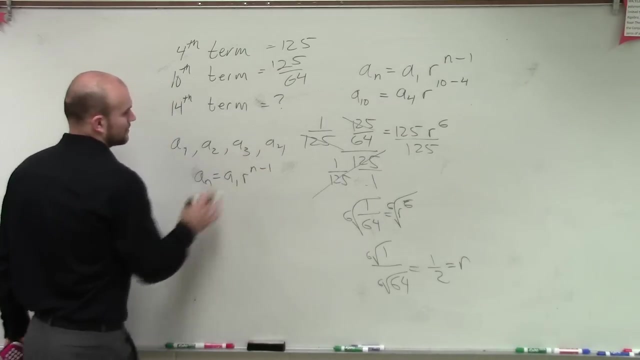 what a sub 1 is going to be. first, Yes, So now we at least figured out what r is right, And that's good. So now sorry. So OK, So we have a sub. n equals a sub 1 times r to the n minus 1, right. 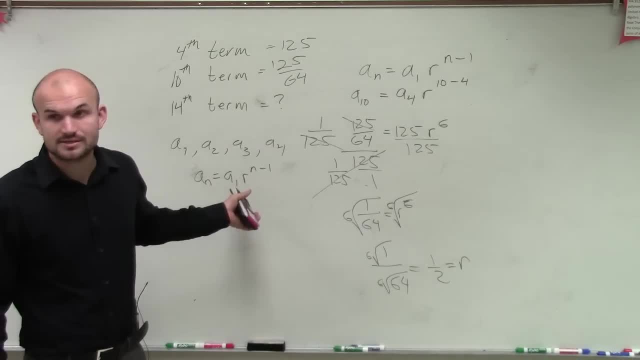 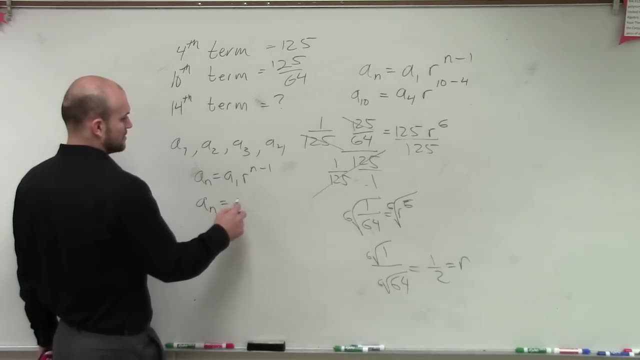 Now what we need to do is be able to figure out what our a sub 1 is. Yes, Yes, So we have a sub. n equals a sub 1 to the 1 half times n minus 1.. OK, Put it in there. 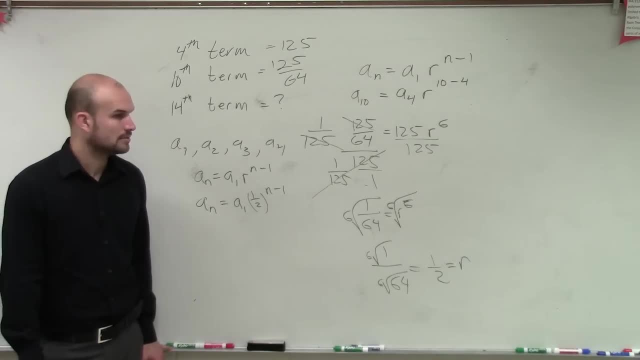 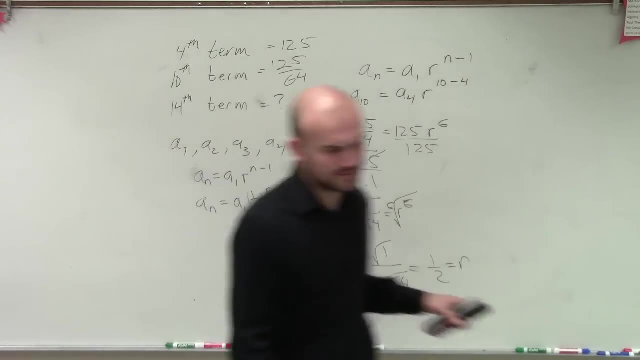 Why do you need to put 1 minus 1?? Because that is not what we're trying to solve, for No, We're trying to find out our rule. Our rule, Yeah. Which problem do I have to work with? So why can't you put it in? 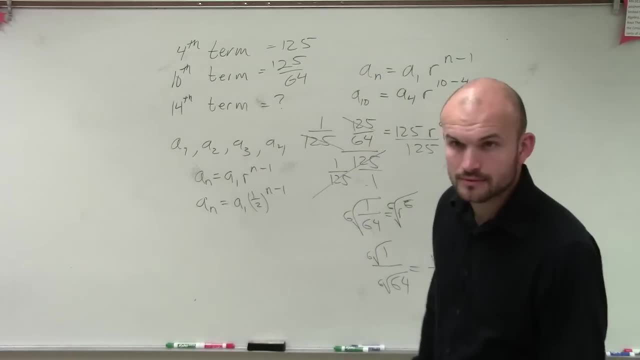 Huh, Why can't you put n to the n, Like put n? I don't know, You never understand. Just keep going, I'll see what you get. I hear what I'm asking. Well, looking at this, we're going to have to figure out. 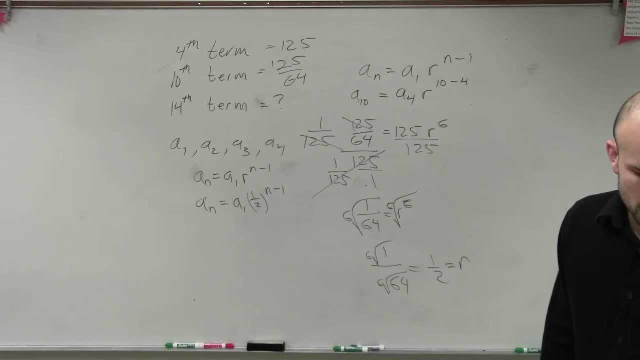 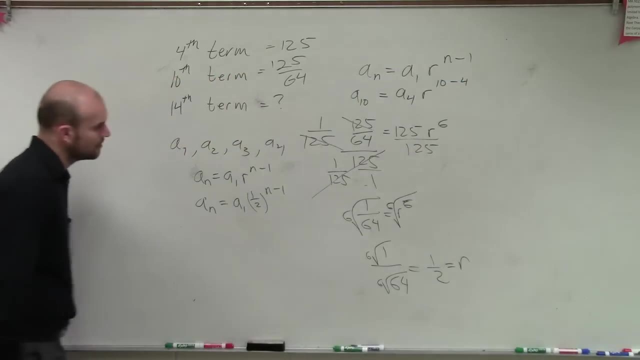 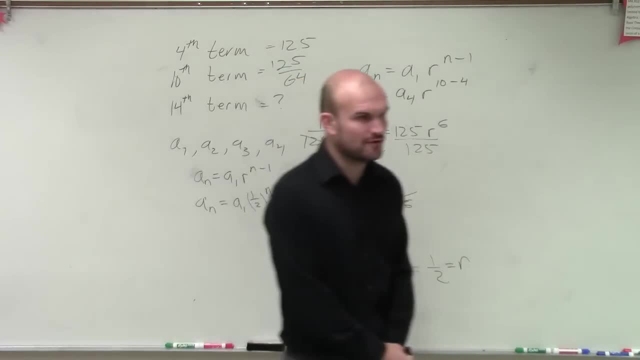 I'm having an issue with it, right, Because how am I going to really be able to find out my rule, how to be able to solve for a sub 1 because or 8, how am I going to be able to solve for my a sub 1, which is this: 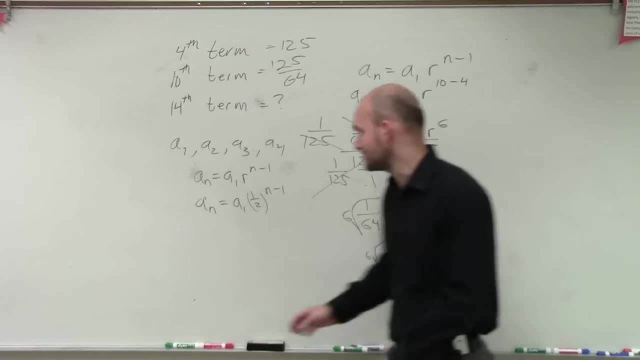 And I still don't even know what my value of n is, So it's not going to work like my arithmetic sequence. Wait, But you had it as 10 and the other one. What is 10?? Oh, I see what you're saying. 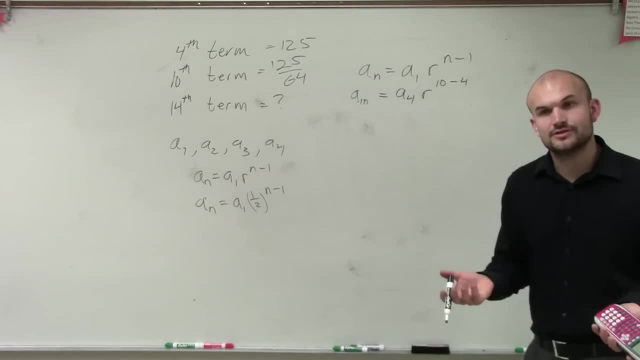 OK, But what I can do though, Yeah, why wouldn't you put 1 in? Well, listen, We can do this. the same thing, though. What I was trying to do is like arithmetic: you can go back to your original points and figure it out. 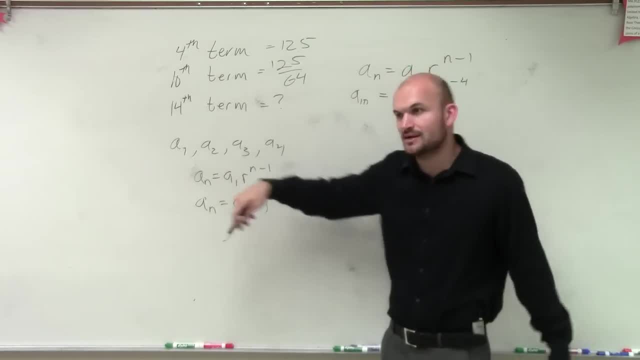 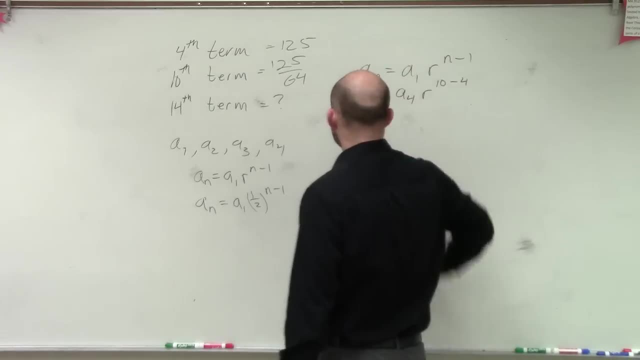 But we can't do that in this case, right, We can't figure out what it is. However, I could do this. If I say a sub n equals a sub 1.. I already have that written down. What if I started? I need to figure out what the 14th term is. 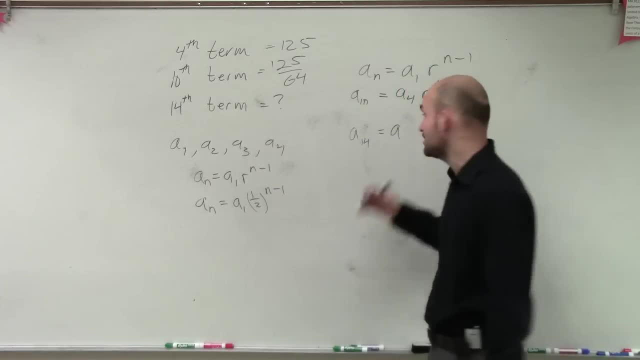 I know what the 10th term is. I don't know what the first term is, but I know what the 10th term is And I know what my r is, which is 1 half Right. I'm sorry, let's just do r. 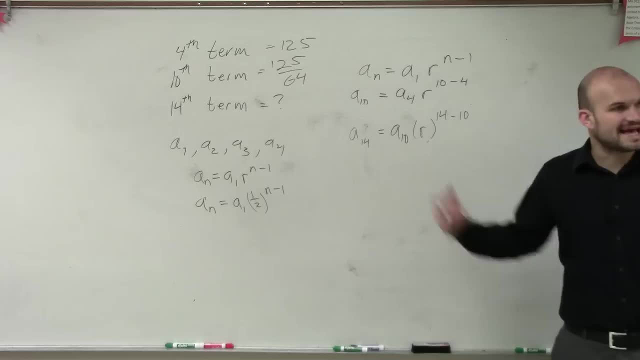 And I know I can do 14 minus 10.. Is that something I could plug in that will tell me what a to the 14th is? Because I know what 10 is and I know what 14 minus 10.. And I know a sub 10,, I know r and I can do 14 minus 10.. 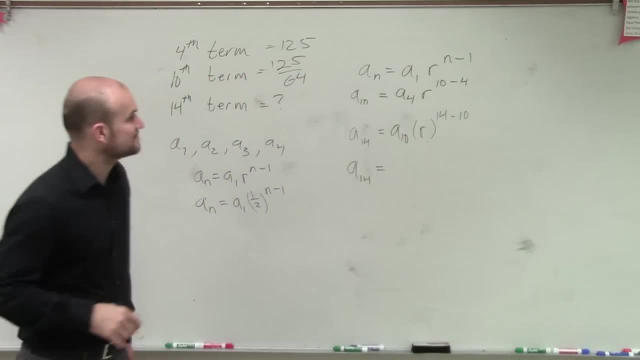 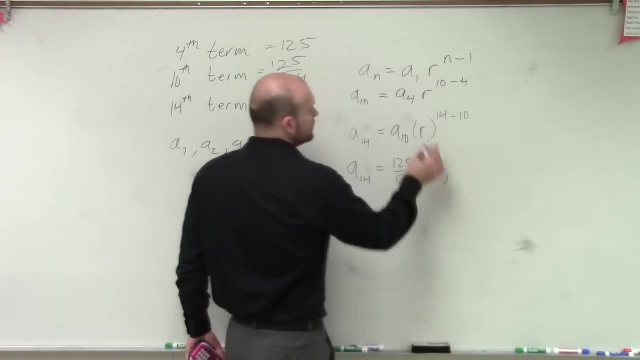 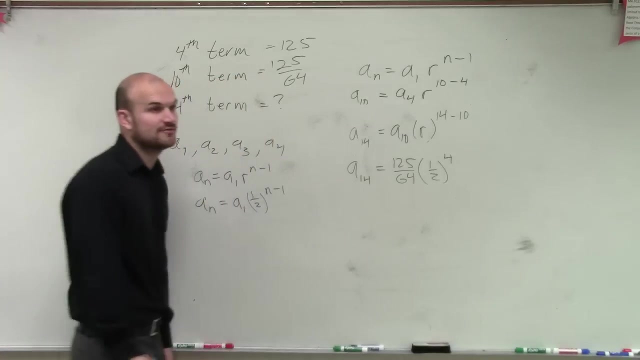 So therefore I could say a sub 14 equals a sub 10, which we said was 125 over 64, times 1, half raised to the 4th power And 1 half raised to the 4th power. So 4 raised to the 4th power is going to be 1 over 16.. 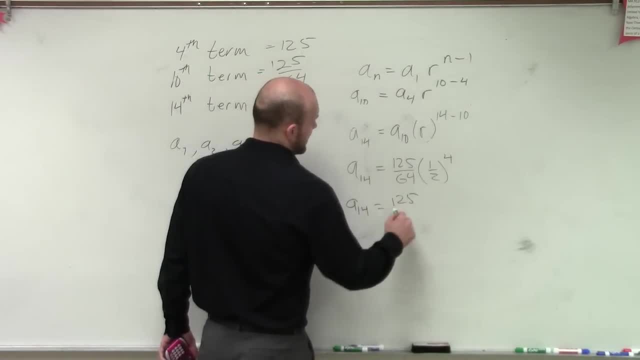 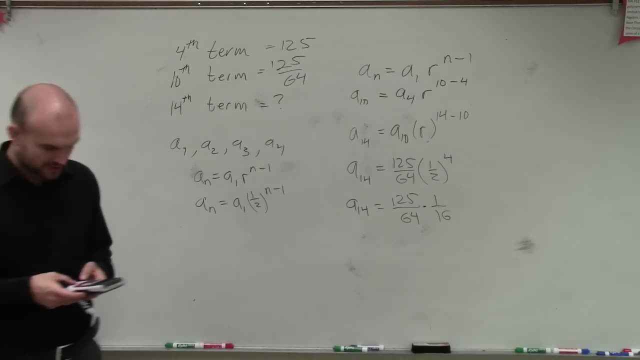 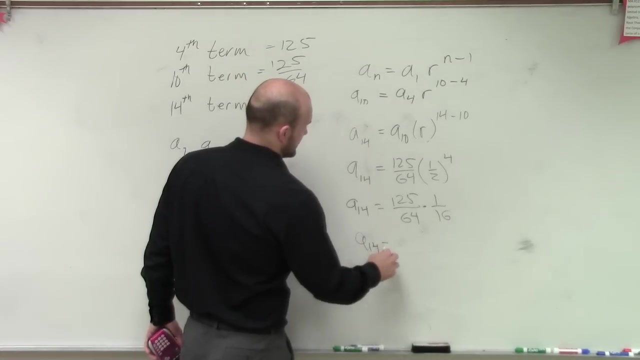 So we have a to the 14th equals 125 over 64, times 1 over 16.. So I just do 64 times 16, and 1,024.. So a sub 14 equals 125 over 1,024.. 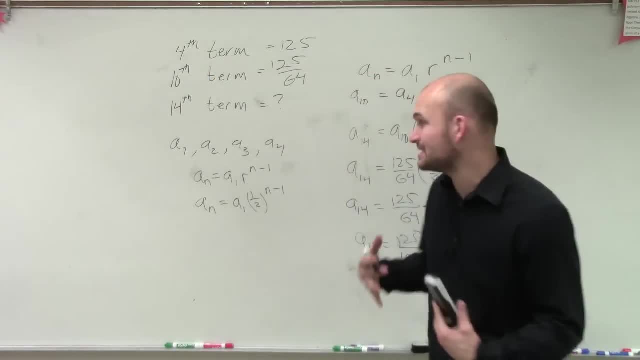 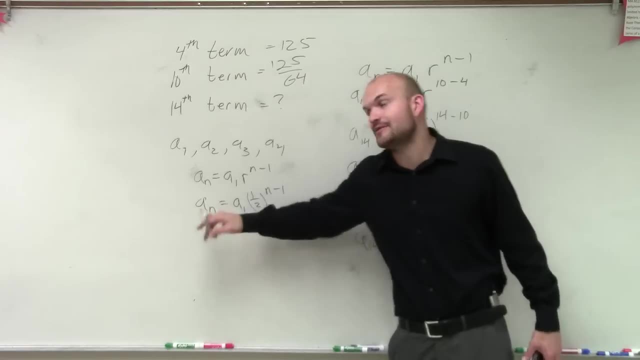 So what I wanted to show you is: we don't always have to go back to use this formula to find a sub 1.. You don't have to go back and find the formula to go to a sub 1.. If you know your value of 10, right, and you want to find 14,.